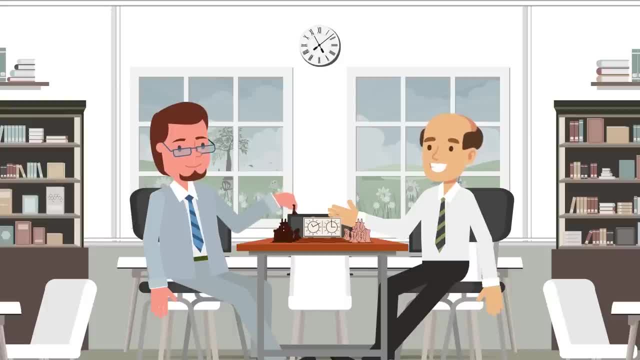 he collaborated with economist Oskar Morgenstern on a book called The Theory of Games and Economic Behavior in 1944.. The Library of Economics and Liberty EconLib states that in their book, von Neumann and Morgenstern asserted that any economic situation could be defined as the 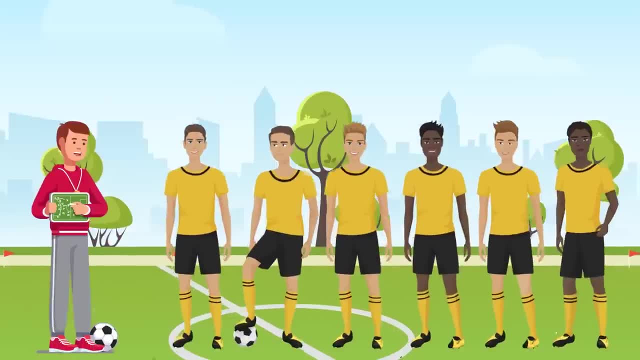 outcome of a game between two or more players. What is a game according to Game Theory? Yale economics professor Ben Pollack notes: a game-hunting game theory is a game in which two or more players play a game. The game theory is a game in which two or more players play a game. The game theory is a game. 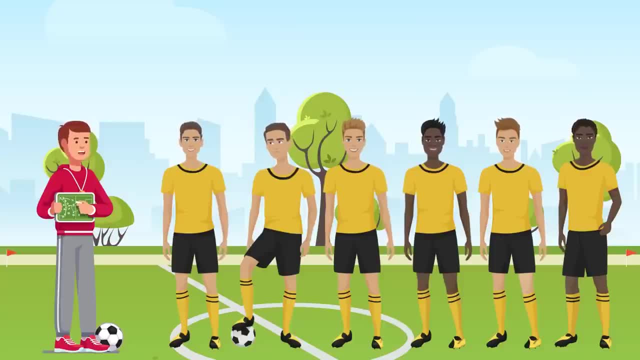 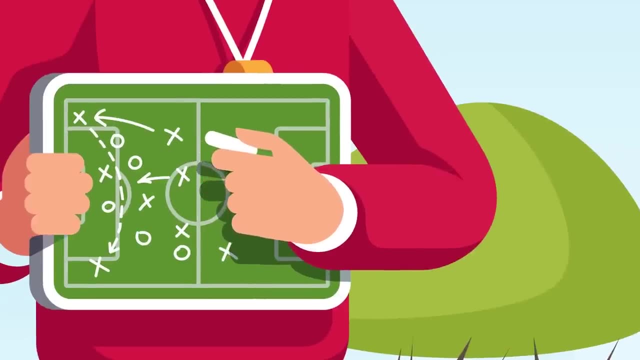 has three basic components-: players, strategies and payoffs. As we just mentioned, game theory applies to games involving two or more players. In a game, players share common knowledge of the rules, available strategies and possible payoffs of the game. However, it is not always the case. 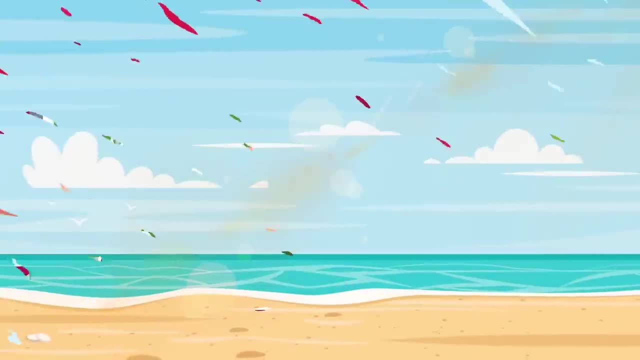 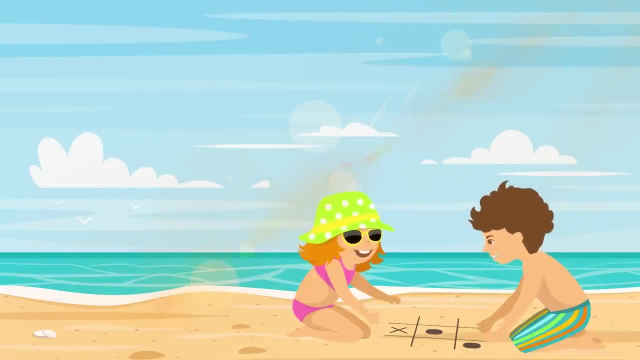 that players have perfect knowledge of these elements of a game. Strategies are the actions that players take in a game. Strategy is at the heart of game theory. Forbes describes the theory presented in A Theory of Games and Economic Behavior as the mathematical modeling of a strict 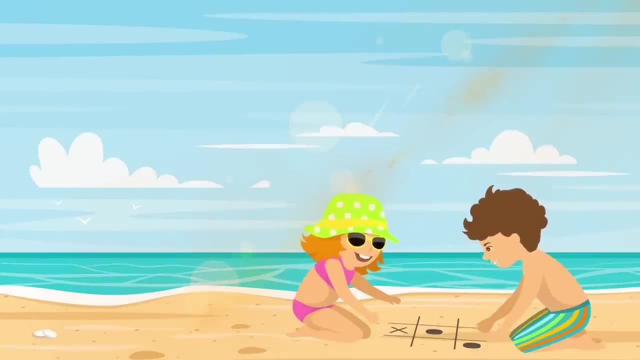 interaction between rational adversaries, where each side's actions would depend on what the other side would do. The concept of strategic interdependence- the actions of one player influencing the actions of other players- is one important aspect of von Neumann's version of game. 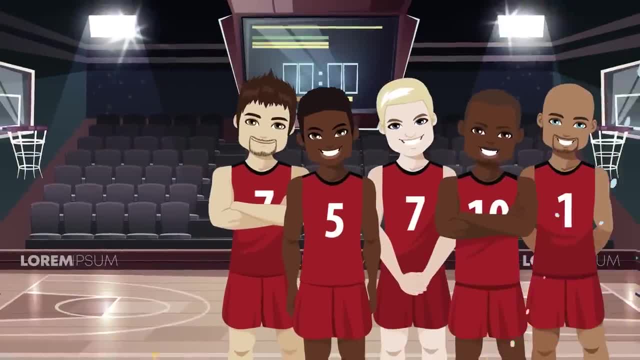 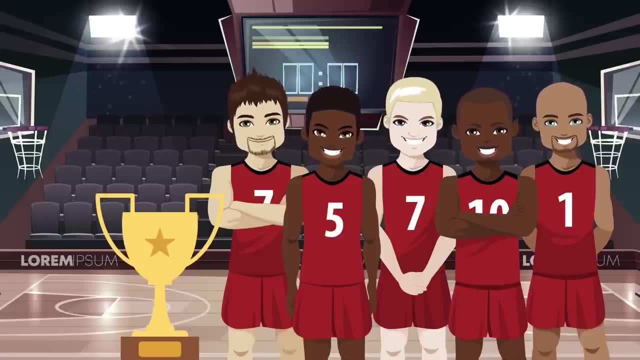 theory that is still relevant today. And then there are payoffs, which one source describes as the outcome of the strategy applied by the player. Payoffs could be a wide range of things, depending on the game. It could be profits, a peace treaty or getting a great deal of money. 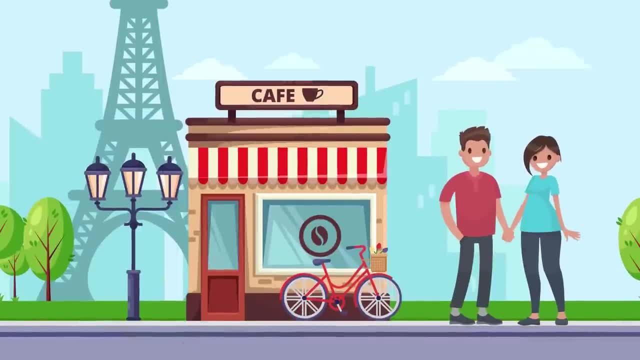 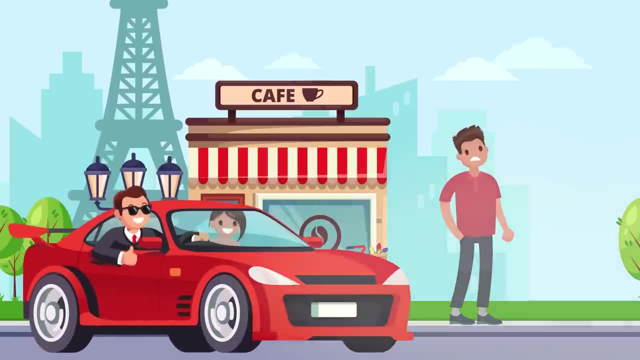 One limitation of von Neumann's version of game theory is that it focused on finding optimal strategies for one type of game called a zero-sum game. In a zero-sum game, one player's loss is the other player's gain, according to Forbes. Another source notes that players can neither. 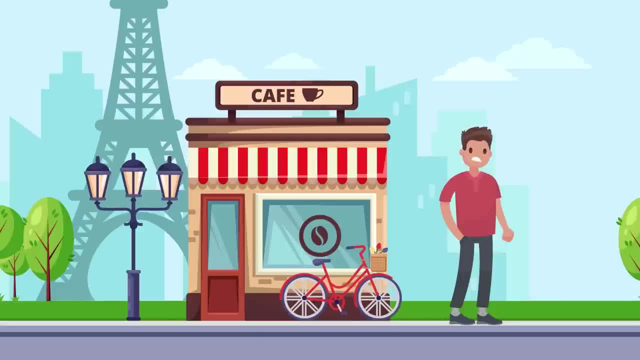 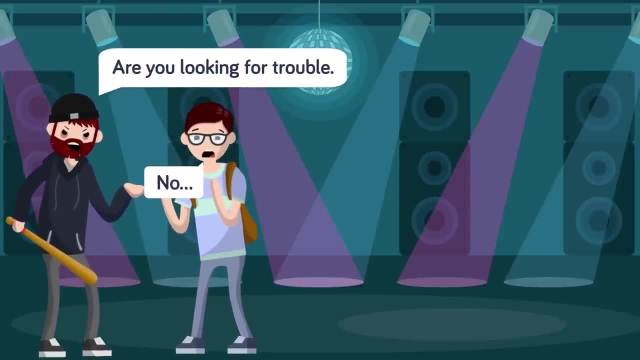 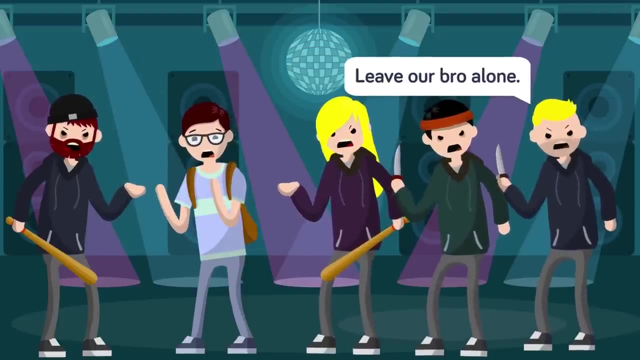 increase nor decrease the available resources in zero-sum games. Critics have noted that life is not often as simple as a zero-sum game. More complicated game scenarios are possible in the real world. For example, players can do things like find more resources or form coalitions that increase the gains of several players. 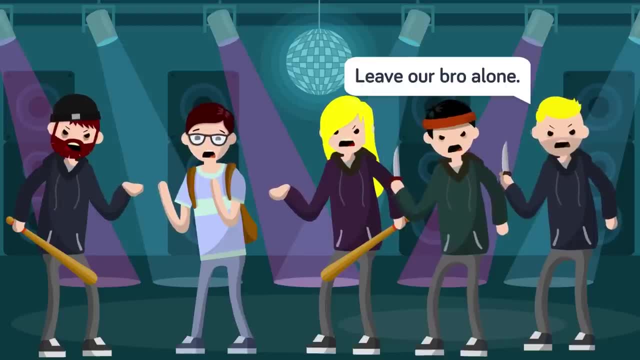 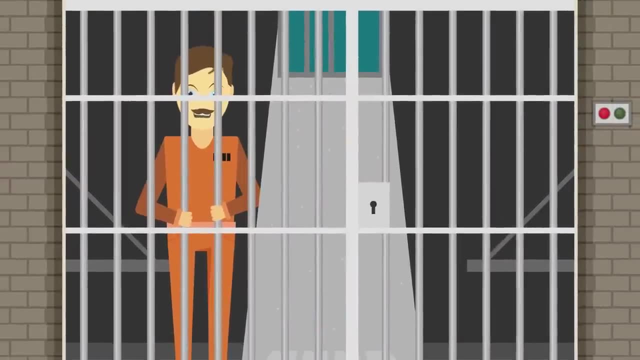 Game theory has evolved to analyze a wider range of games, such as combinatorial games and differential games, but we have to look at only one. A classic example of a game often studied in game theory is called The Prisoner's Dilemma. Different versions of this game are: 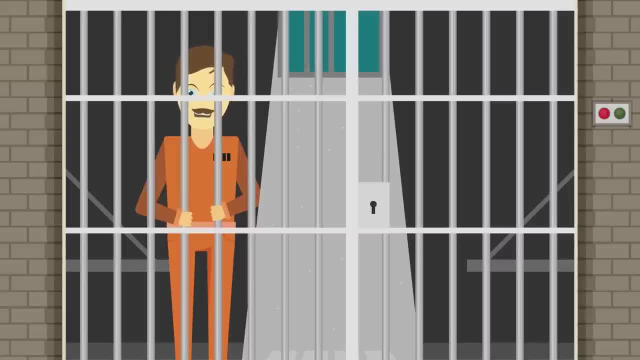 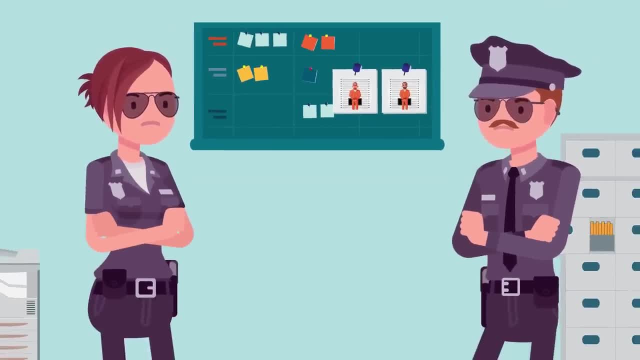 available on the internet. This version is from the Fundamental Finance website. There are two prisoners, Jack and Tom, who have just been captured for robbing a bank. The police don't have enough evidence to convict them, but know that they have committed the crime. They put Jack and Tom in separate interrogation. 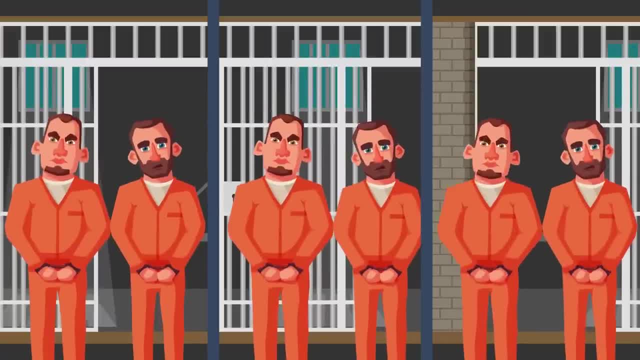 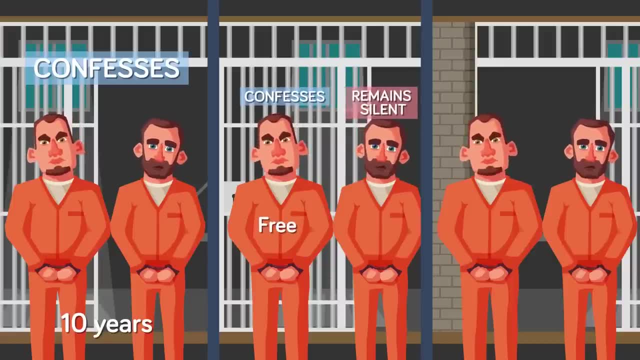 rooms and lay out the consequences. If both Jack and Tom confess, they will each get ten years in prison. If one confesses and the other doesn't, the one who confessed will go free and the other will spend twenty years in prison. If neither person confesses, they 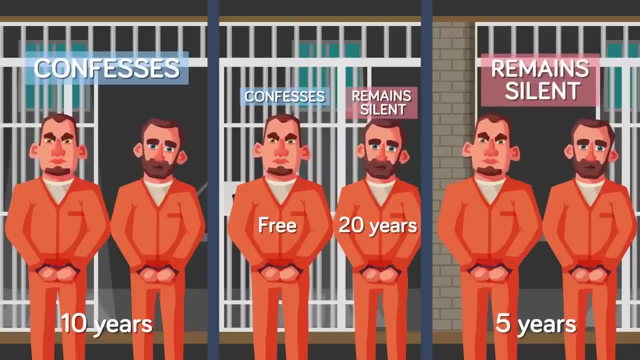 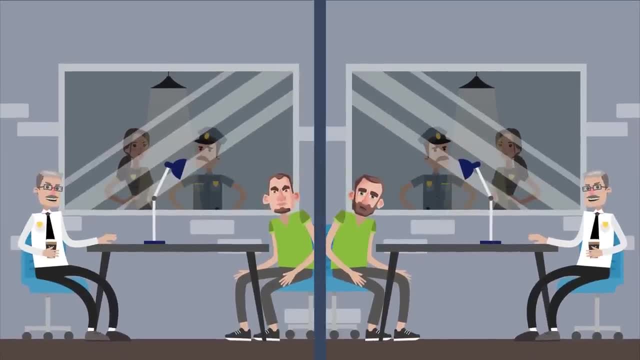 will both get five years for a different crime they were wanted for. The Prisoner's Dilemma contains the basic elements of a game. The two players are Jack and Tom. There are three strategies available to them: confess or don't confess. The payoffs of the 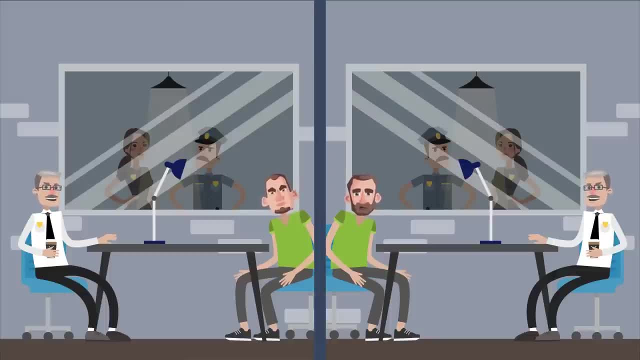 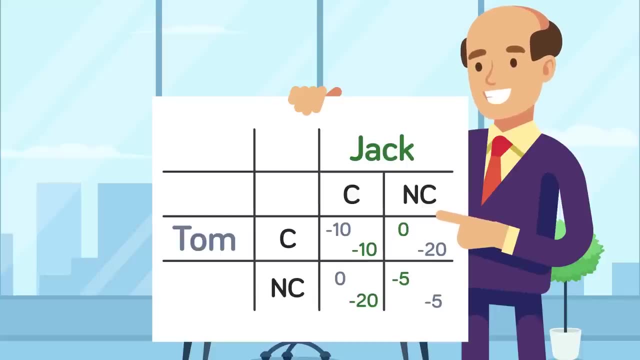 game range from going free to serving five, ten or twenty years in prison. As Fundamental Finance explains, it's easier to see and compare these outcomes or payoffs if they are put into a matrix, Since Tom's strategies are listed in rows or the x-axis. 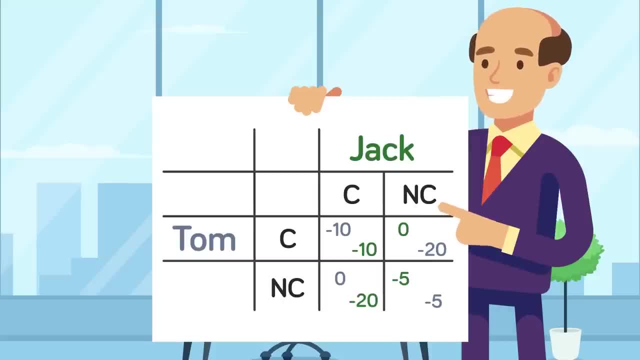 his payoffs are listed first. Jack's payoffs are listed second because his strategies are in columns or on the y-axis. C means confess and NC means not confess. This matrix is called normal form in game theory. Moves are simultaneous, which means that neither player knows the 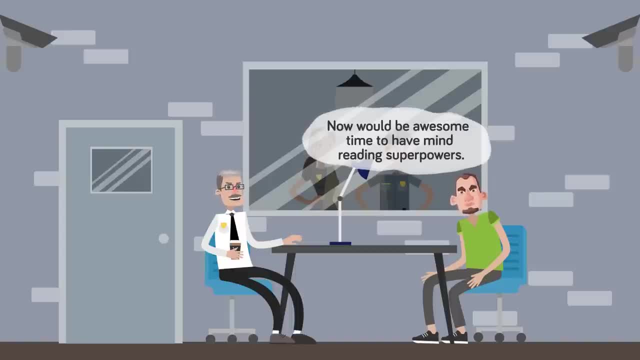 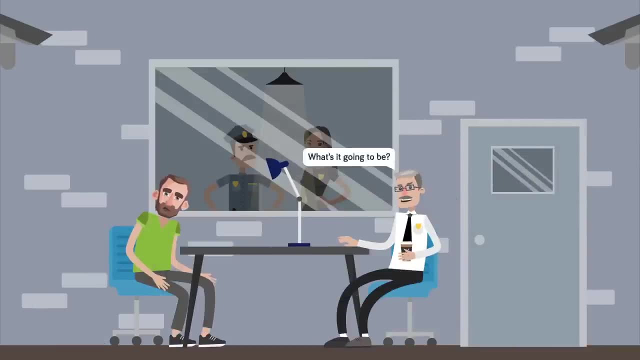 other's decisions, and decisions are made at the same time. In this example, both prisoners are in separate rooms and won't be let out until they have both made their decisions. One common solution to simultaneous games is known as a dominant strategy. Fundamental Finance defines it as the strategy that has the best payoff, no matter what the other player. 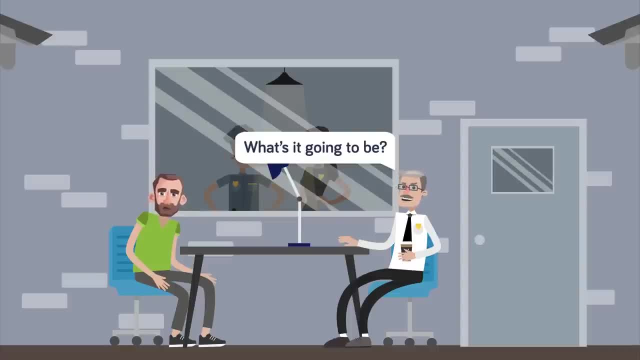 chooses. Tom does not know if Jack will confess or not. He takes a look at both options. If Jack confesses and Tom does not, Tom will get twenty years in prison. If both Jack and Tom confess, Tom will only get ten years. If Jack does not confess and Tom does, Tom 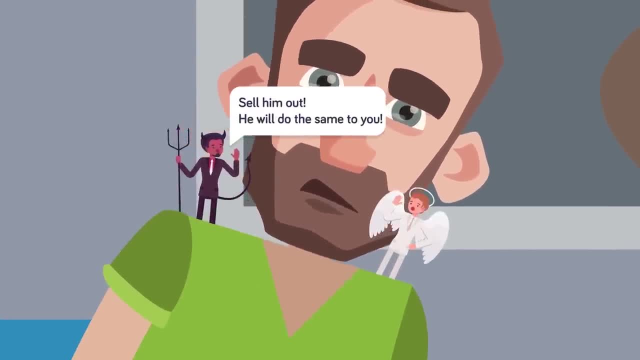 will go free. The best strategy for Tom is to confess, because it leads to the best payoff, regardless of Jack's actions. Confessing will cause Tom to either go free or serve less prison time than if he did not confess. Jack is in the same situation and has the same 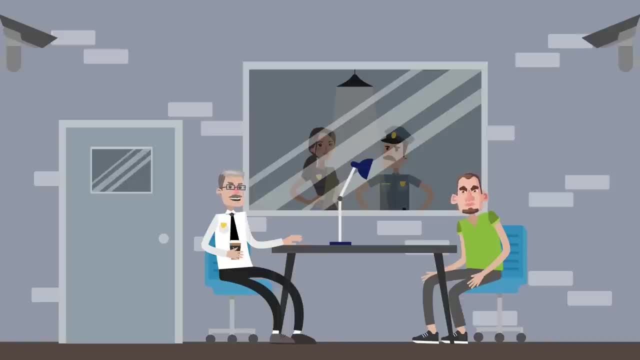 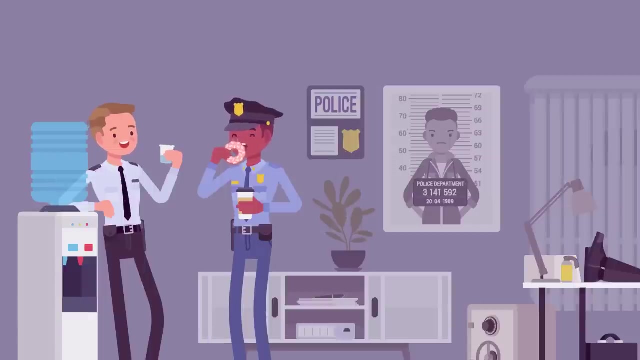 option as Tom. As a result, the best strategy for Jack is to also confess, because it leads to the same best payoffs that Tom will get. One economics website states that a dominant strategy equilibrium is reached when each player chooses their own dominant strategy. Why is the strategy of both not confessing? 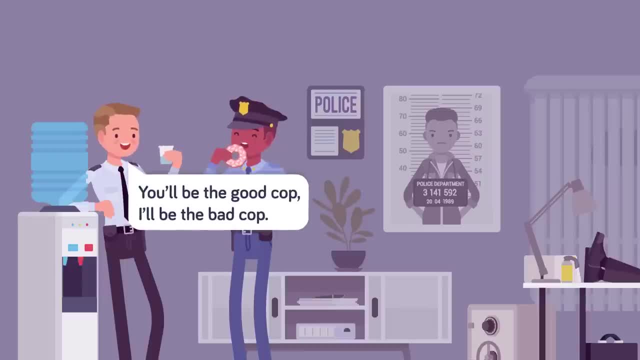 not the best choice. While this option would give both of them less time in prison than if they confessed, it would only work if each of them could be sure the other one would not confess. It is unknown whether Tom and Jack would be able to work together with that. 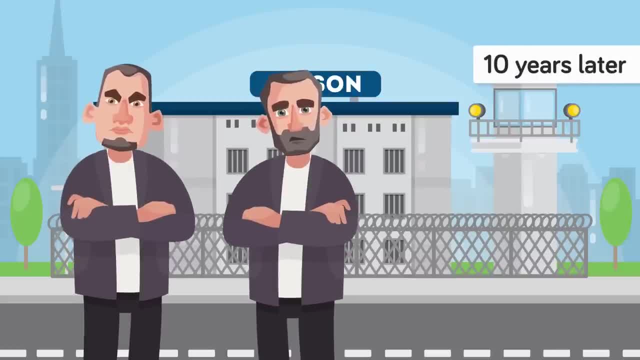 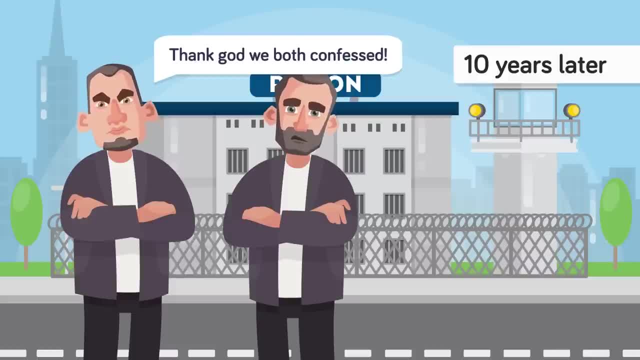 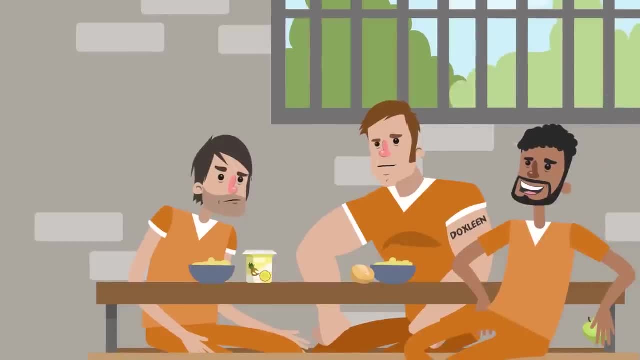 of not confessing because it has greater penalty than they would if they confessed. Confessing also gives each of them the possibility of serving no prison time, which is even less than five years in prison. The Prisoner's Dilemma is a good example of how rationality can be problematic in game. 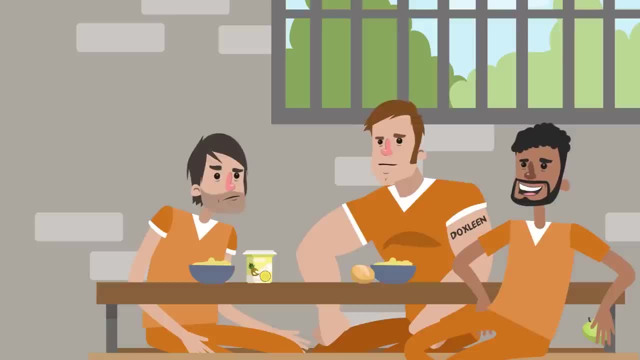 theory University of British Columbia, Vancouver, researcher Yamin Hatun calls it one of the most debatable issues in game theory. Hatun points out that almost all of the theories are based on the assumption that agents are rational players who strive to maximize the utilities or payoffs. Yet studies demonstrate that players do not always act rationally. 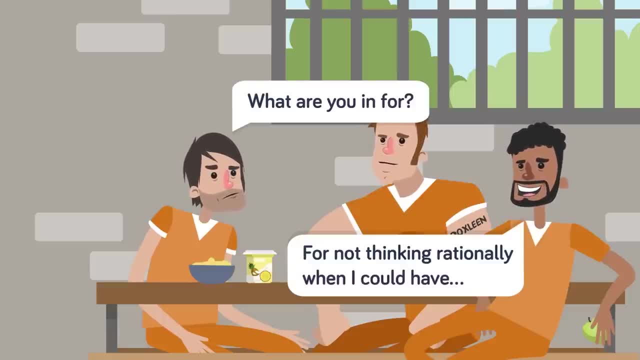 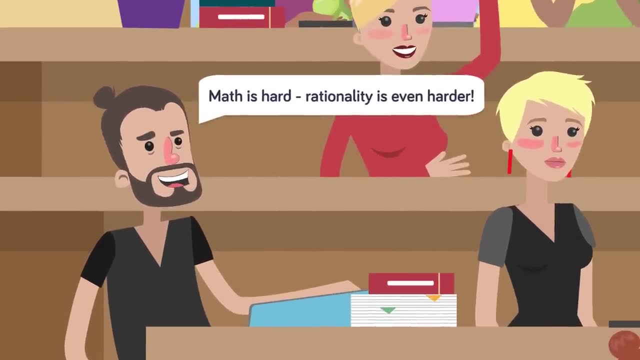 and that the conclusions of rational analysis sometimes fail to conform to reality, As we can see from this game. the most rational strategy that would give both players less prison time was not the best choice, while a choice that involves both players doing more prison time was. 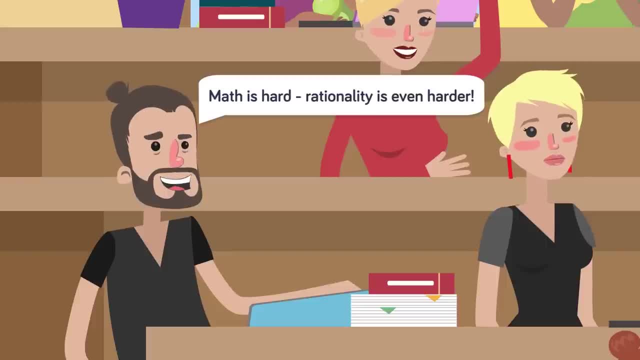 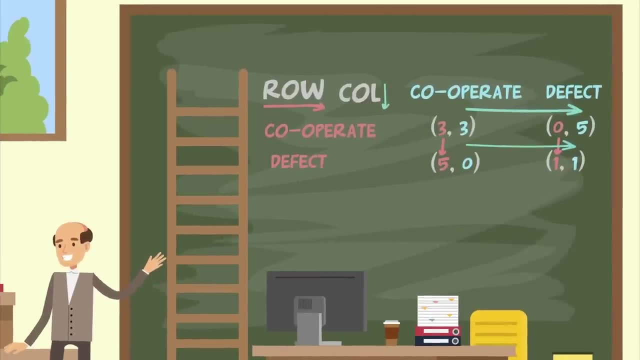 The Prisoner's Dilemma also reflects how other game theorists were able to fix some of the problems with von Neumann's version of game theory. One of them was mathematician John Nash. He found a way to determine optimal strategies for any finite game. A New Yorker 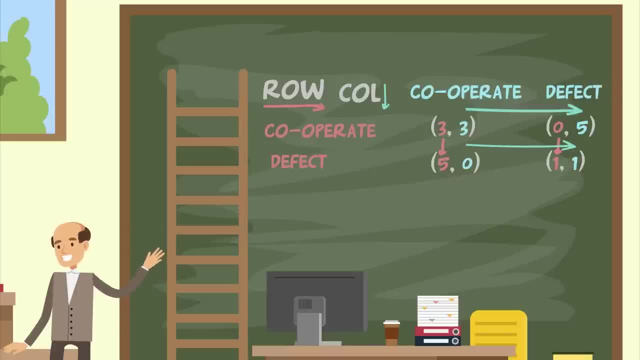 article describes the Nash Equilibrium as a particular solution to games, one marked by the fact that each player is making out the best he or she or it possibly can, given the strategies being employed by all of the other players When Nash Equilibrium is reached. 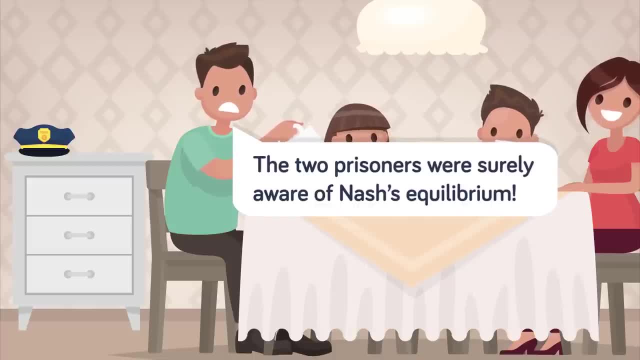 into game. none of the players wants to change to another strategy, because doing so will lead to a worse outcome than the current strategy. In The Prisoner's Dilemma, the Nash Equilibrium's strategy is based on the assumption that both players have the right to choose what they. want to do and what they don't want to do In the Prisoner's Dilemma. the Nash Equilibrium's strategy is based on the assumption that both players have the right to choose what they want to do and what they don't want to do. The Nash Equilibrium is the strategy. 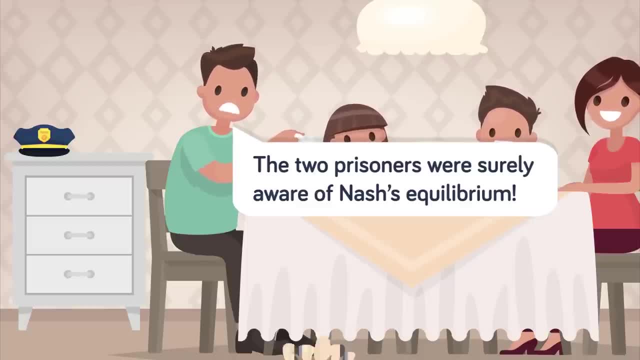 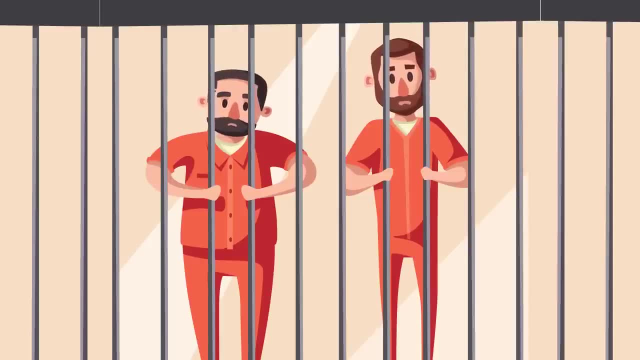 of both players confessing there is no other, better option for either player to switch to. From this game we can see another interesting aspect of the Nash Equilibrium. Mathematician Istok Hozo points out that any dominant strategy equilibrium is also a Nash. 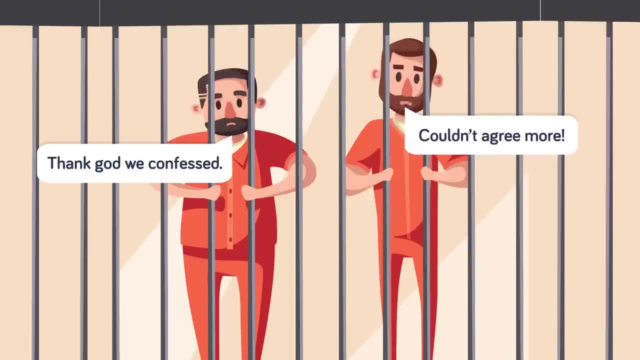 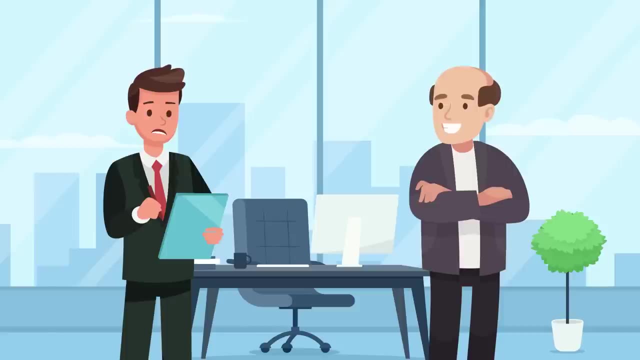 Equilibrium. He explains that this is because the Nash Equilibrium is an extension of the concepts of dominant strategy equilibrium. However, he notes that the Nash Equilibrium can be used to solve games that don't have a dominant strategy. Nash received great praise for the Nash Equilibrium and for his other works in game theory, but not from John. 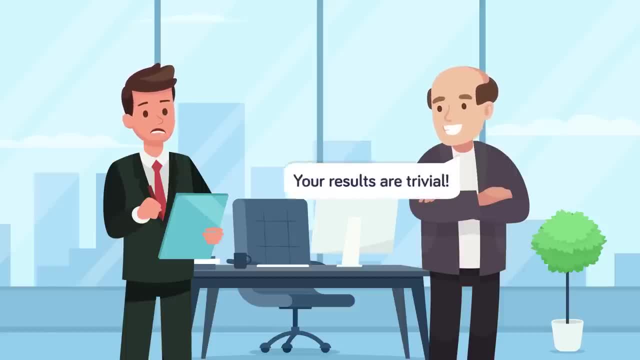 von Neumann. According to Forbes, von Neumann, consumed with envy, dismissed the young Nash's result as trivial, meaning mathematically simple. Others did not share in von Neumann's assessment of Nash's work. Nash, Reinhardt Selton and John Harsanyi went on to share. the 1994 Nobel Memorial Prize in Economic Studies for their work in game theory. When Nash died in 2015, one academic news website summed up his accomplishments this way: Nash's fundamental contribution to game theory was in opening the field up to a wider range of 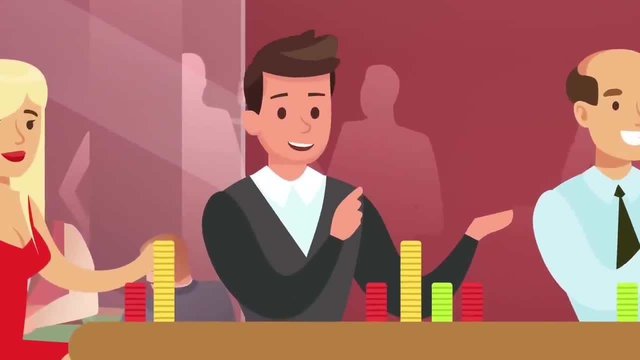 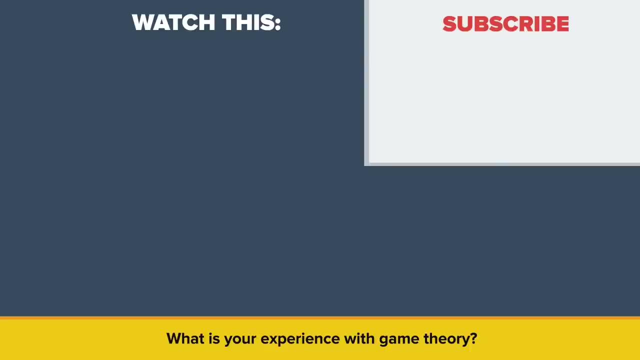 applications and different scenarios to be studied. Without his breakthrough, much of what followed in game theory might not have been possible. What's your experience with game theory? Let us know in the comments. Also, be sure to check out our other video called Could Aliens 65 Million Light Years Away From Earth See? 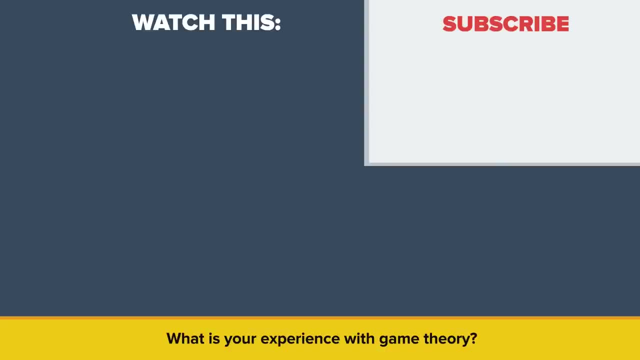 Dinosaurs Alive. Thanks for watching and, as always, don't forget to like, share and subscribe. See you next time. 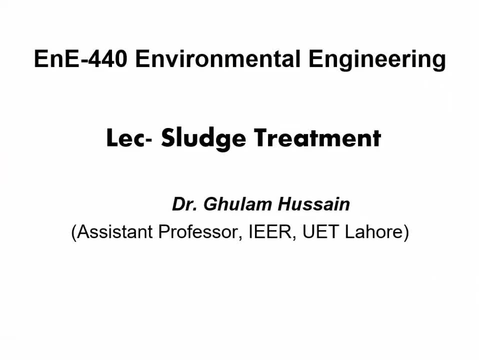 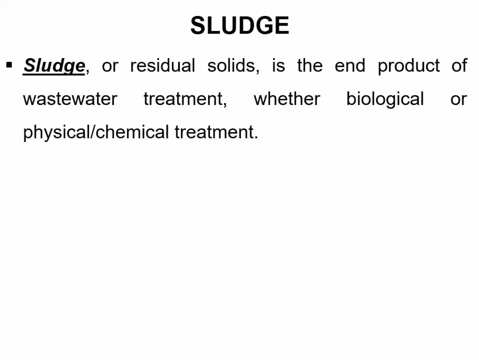 Assalam-u-Alaikum students, Today we are going to discuss about sludge treatment and another very brief topic on site sanitation. Let's first define the sludge, or residual solids. It is the end product of wastewater treatment, whether it is biological or physical or chemical treatment.